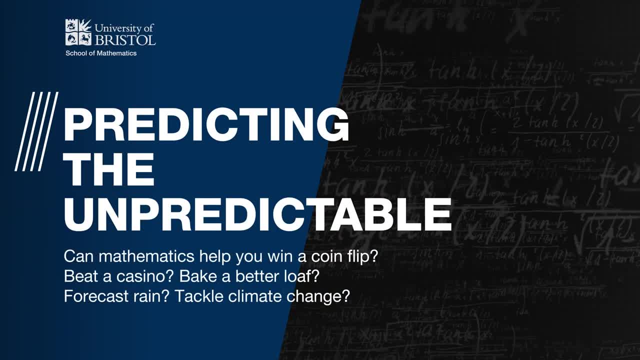 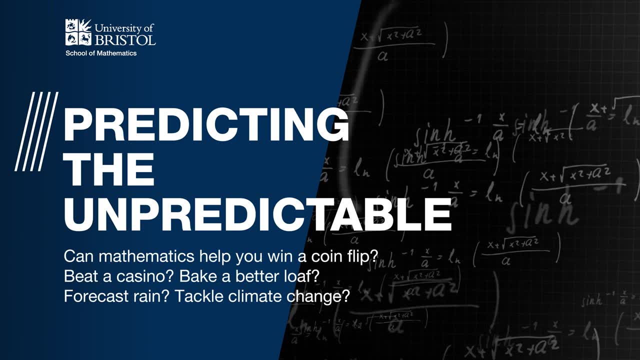 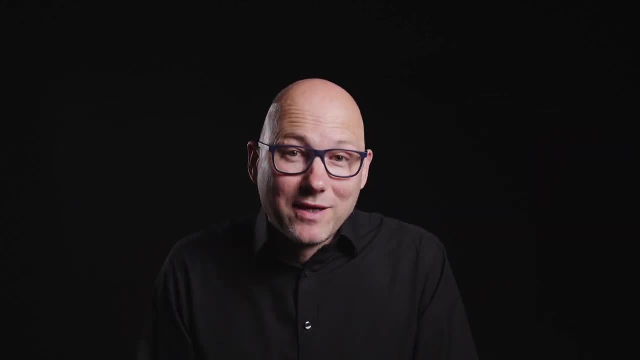 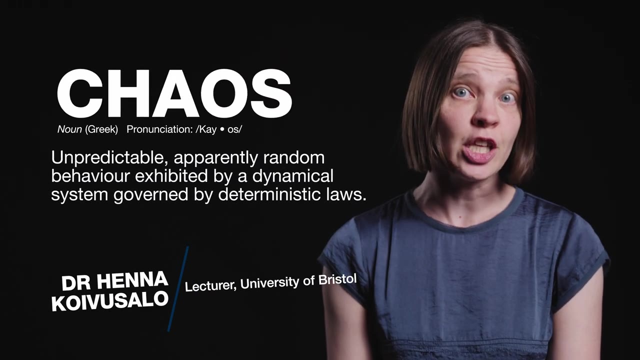 can we really predict the unpredictable? In everyday language, we use the words random and chaotic as if they mean the same thing. However, in a mathematical sense, chaos refers to systems that are extremely sensitive to changes in their initial conditions. Chaotic systems appear random, but in fact behave according. 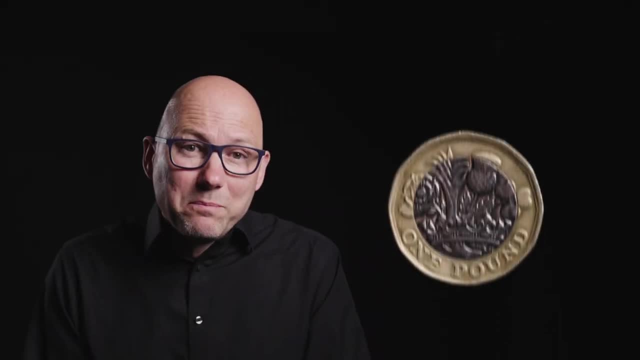 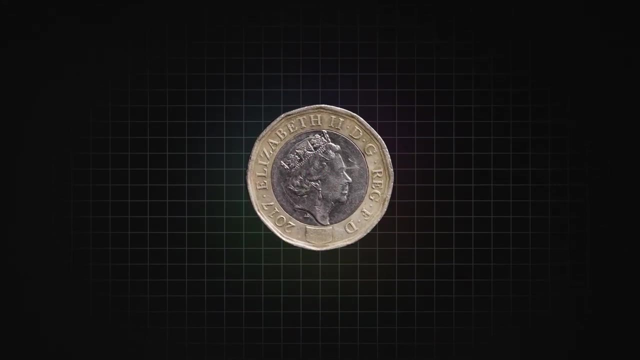 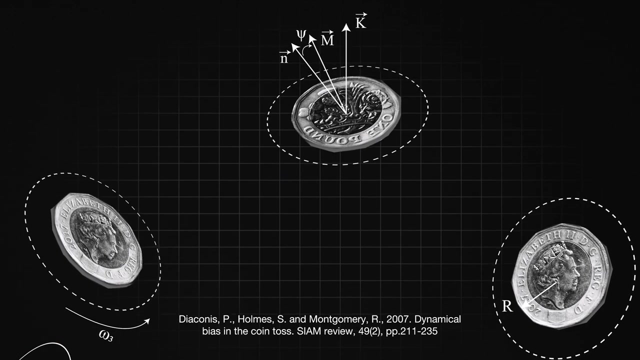 to underlying patterns and rules. An example: The flip of a coin is used everywhere to help us decide things, because the outcome appears to us completely random. However, when a coin is flipped and caught, we know that it will follow Newton's laws of motion exactly So. 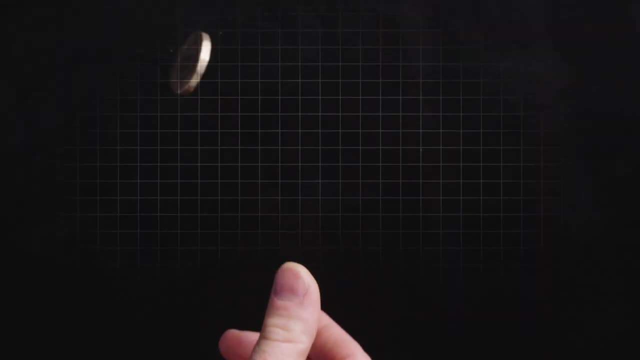 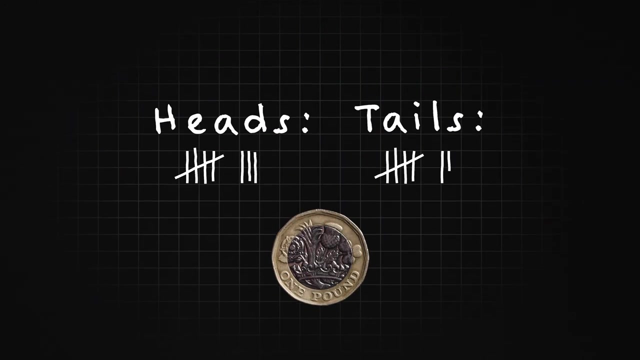 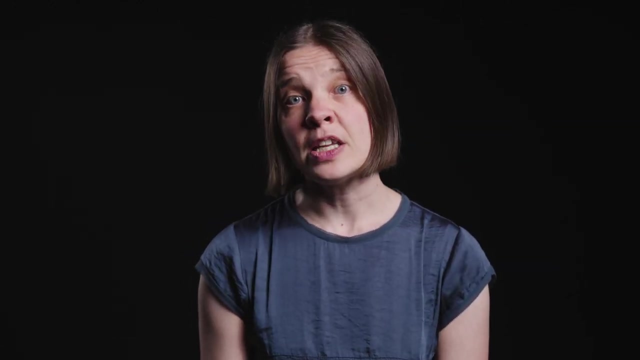 there is really nothing. In theory, if we have enough information about the weight and momentum of the coin, the wind resistance and other variables, we can predict how it will land every time, Though we might not be able to predict the outcome of an individual coin flip or dice roll. 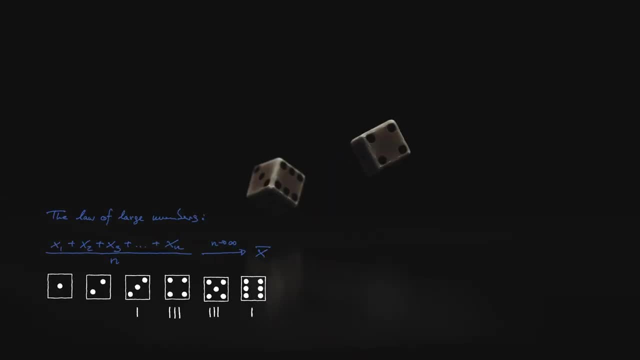 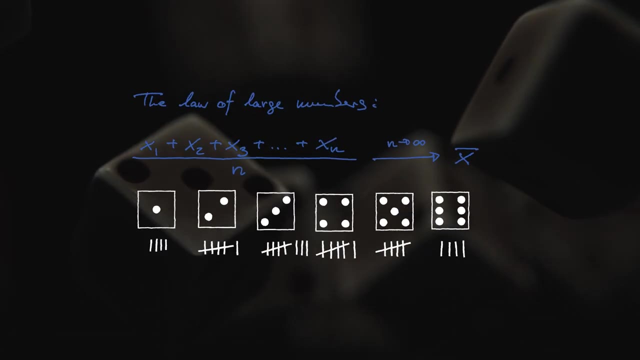 the law of large numbers tells us that if we carry out such actions many times, the average of the results obtained will get closer and closer to the exact values we'd expect. Lotteries and casinos rely on this law every day to ensure that. 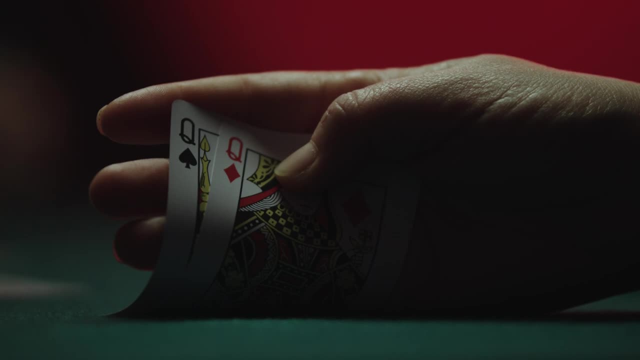 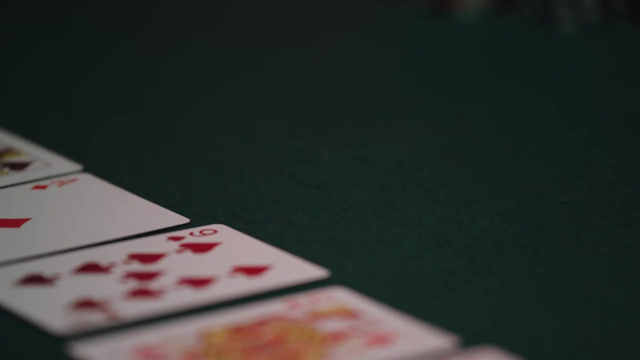 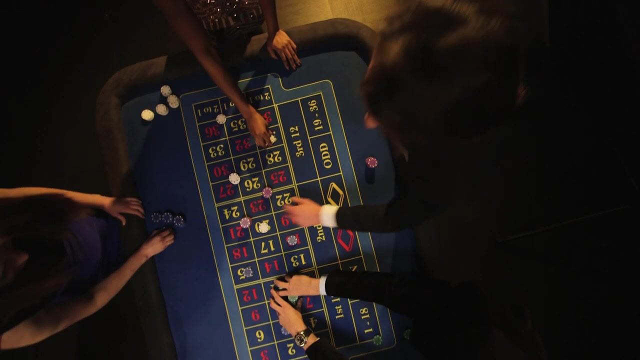 even if gamblers win once or twice, the house always wins eventually. The only way gamblers have ever been able to consistently win at games of chance like roulette is by studying patterns such as physical movement of the wheel or the deceleration of the wheel. 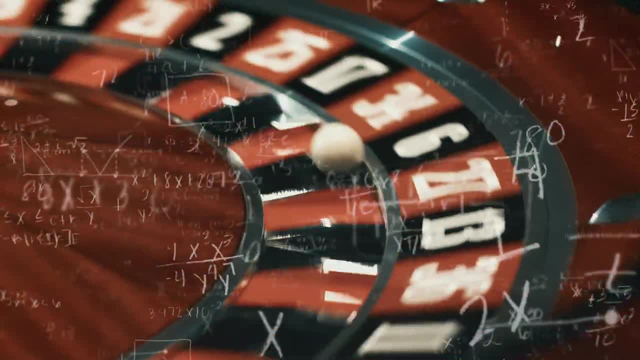 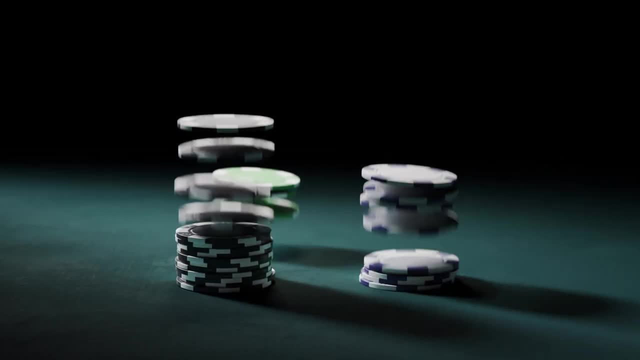 of the ball and using computers in real time to predict the most likely outcomes. In doing so, they shift the probabilities and the law of large numbers to make winning more likely. Of course, casinos are like this because it means they lose money, and so use a variety. 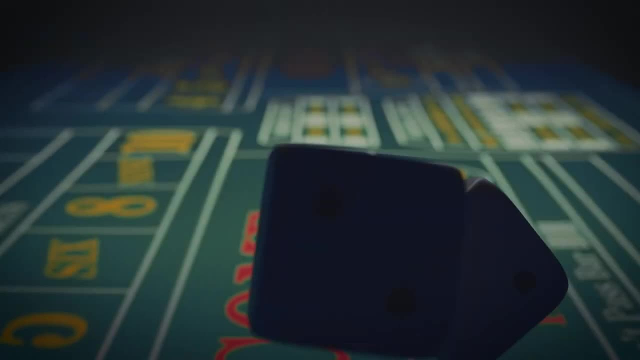 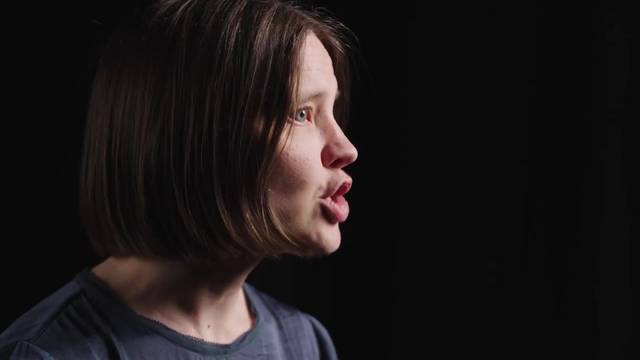 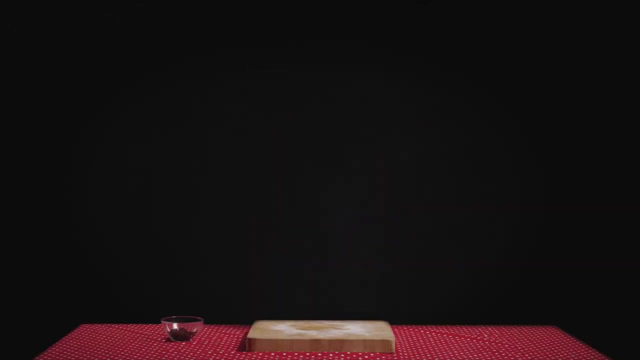 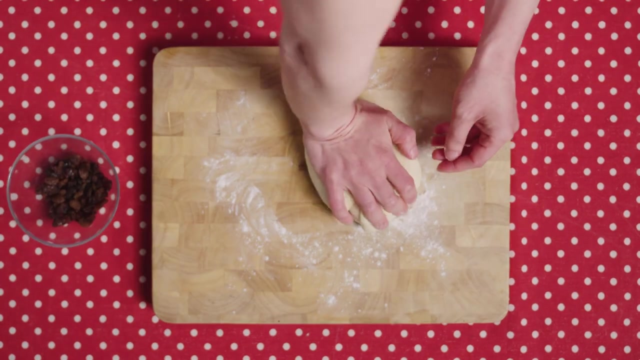 of techniques and modifications to ensure their games remain consistently unpredictable. To better understand how the tiniest changes in the initial conditions of a chaotic system can affect its outcomes dramatically, we can use surprisingly simple examples like a baker kneading dough. As this dough is pressed, folded, turned, pressed and folded again, the distance between 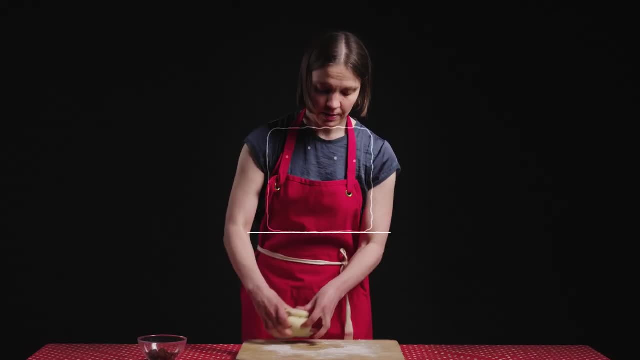 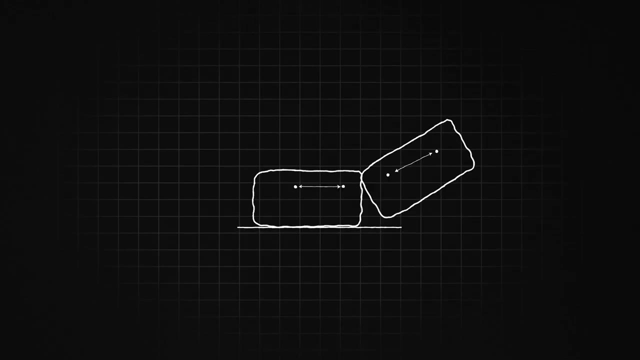 the raisins sprinkled through it increases. As the height of the dough is halved, the horizontal distances between raisins double. If we knead twice, two nearby raisins will be equal. Raisins end up four times as distant, then eight, sixteen, thirty-two and so on. 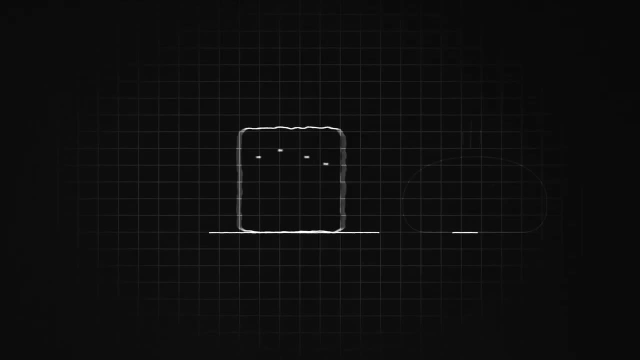 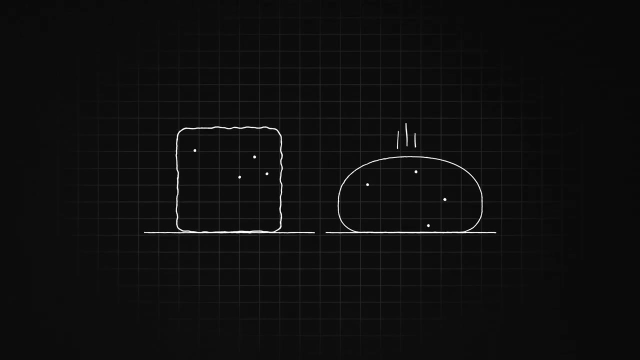 If the starting position of any of our raisins changes even by a millimetre, then the position they end up in will be very different, because the system is exponentially sensitive. Any changes add uncertainty to the system and that uncertainty is amplified exponentially. 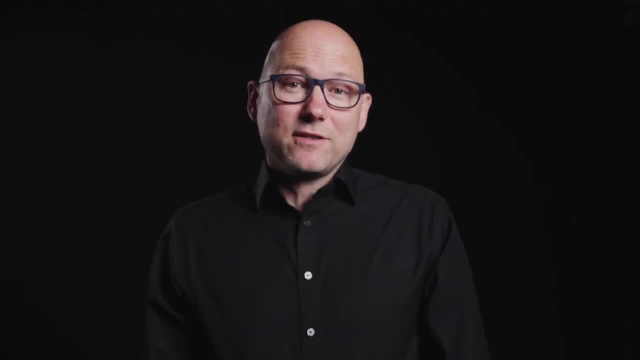 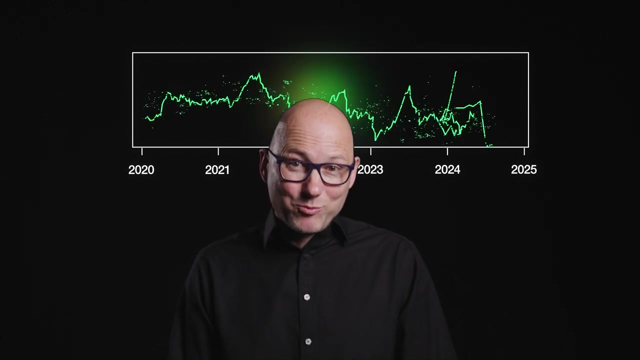 as we knead our dough. A defining characteristic of chaotic systems is that, due to their underlying order, we can predict the outcome of a chaotic system. However, as the effects of tiny changes are amplified exponentially and compounded over time, this breaks down, making longer-term outcomes unpredictable, even with nearly perfect. 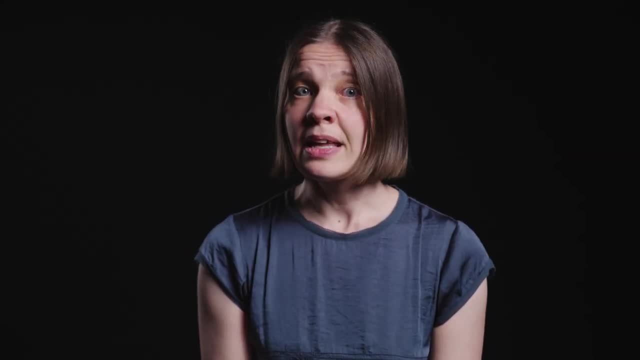 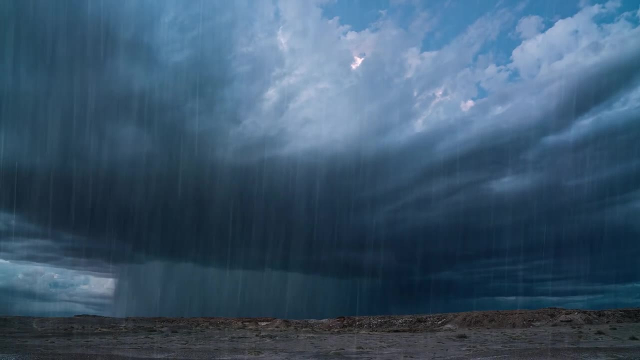 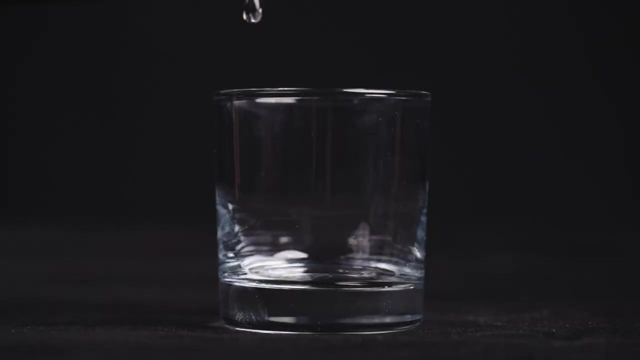 starting information. With hugely complex systems like the weather, you can understand how tiny changes, like a mistake in measuring the temperature at a weather station, can have dramatic impacts on our predictions. All matter in the universe, from coins and dice to oceans and clouds, is made up of microscopic 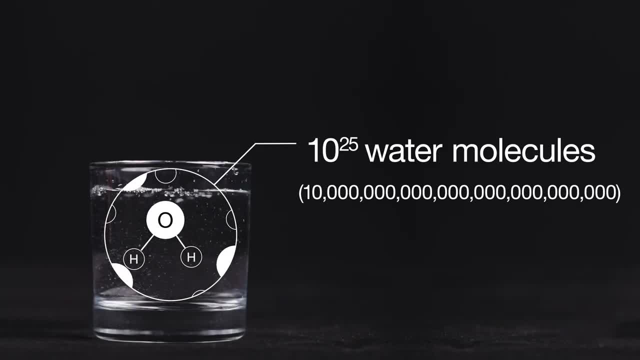 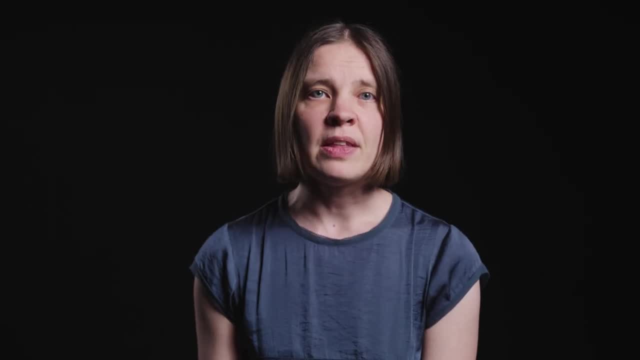 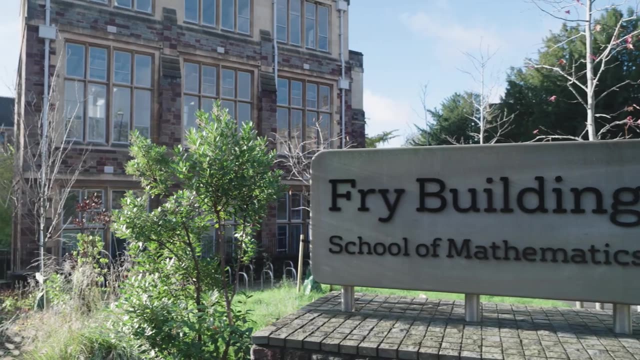 particles, molecules, atoms, electrons and other particles whose microscopic dynamics are governed by the fundamental laws of physics. Characterising the chaos and randomness of microscopic particles and learning to predict their impact at the macroscopic level is one of the key objectives of our research. 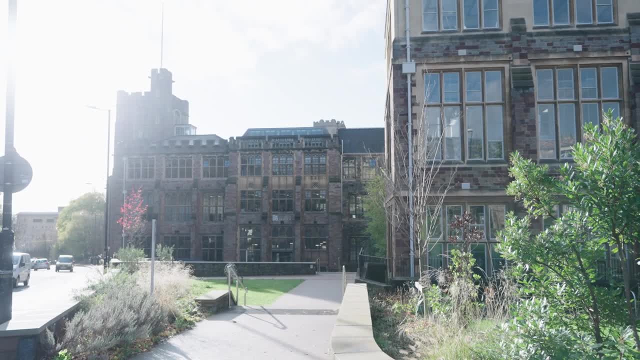 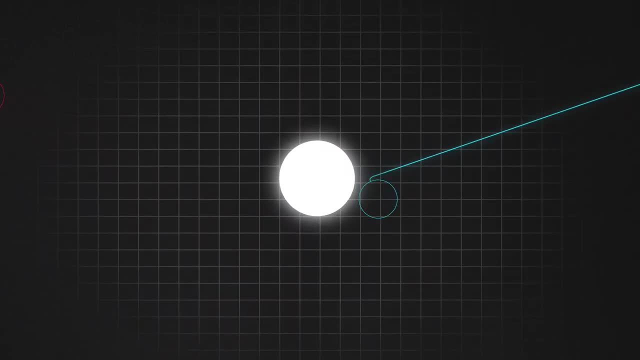 groups here in Bristol, Like raisins in a bowl of dough. Collisions between particles in a gas or fluid show exponential sensitivity to their initial conditions. Just as we can't predict the outcome of a single coin flip or a dice roll, we can't. 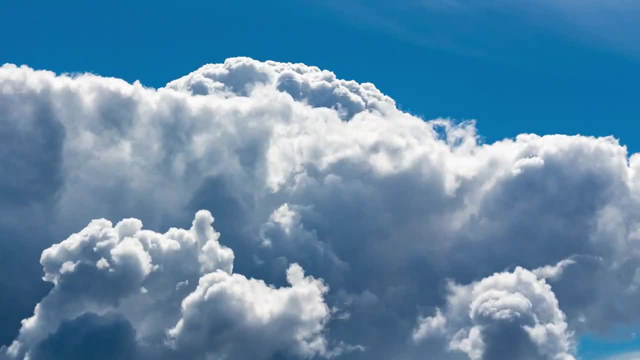 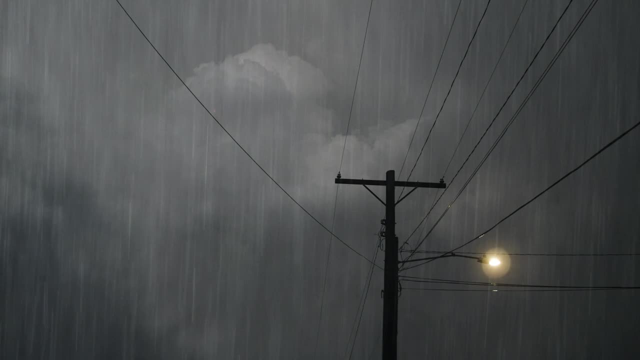 predict the collision of every microscopic particle, but we can again use the law of large numbers and draw on many octillions of collisions to predict what will happen to a gas or fluid at the macroscopic level. Our latest research has used new techniques and pure mathematics to show how an elegant 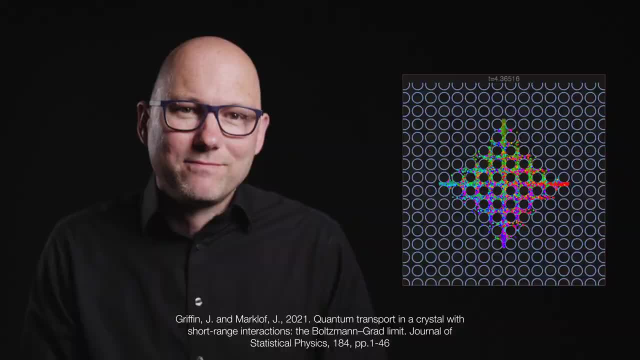 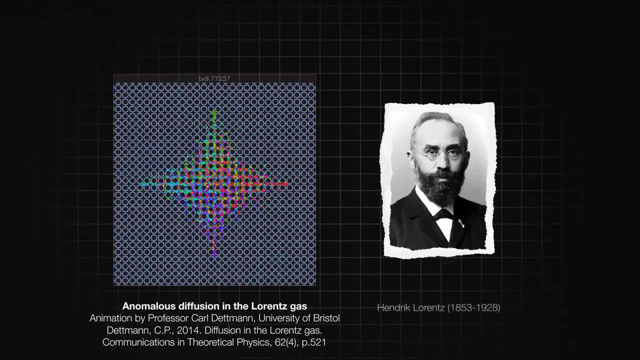 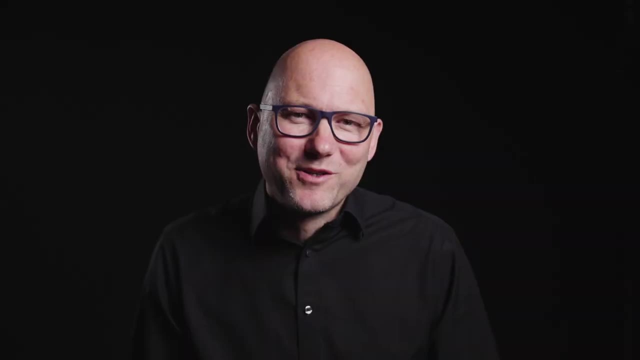 electron gas travels through a crystal lattice. In doing so, we've predicted a new and unexpected transport phenomenon and solved a puzzle posed by Dutch physicist Henrik Lorentz more than a century ago. This brings us a step closer to answering one of the biggest unsolved problems in maths. 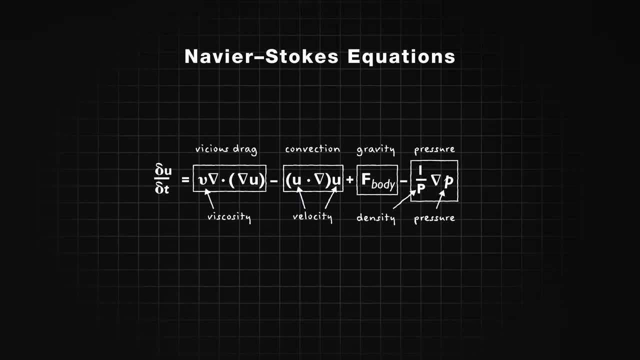 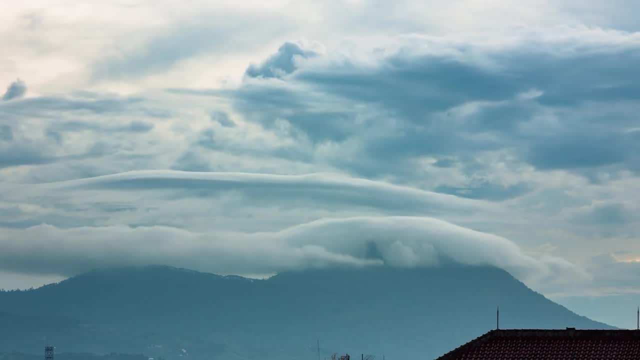 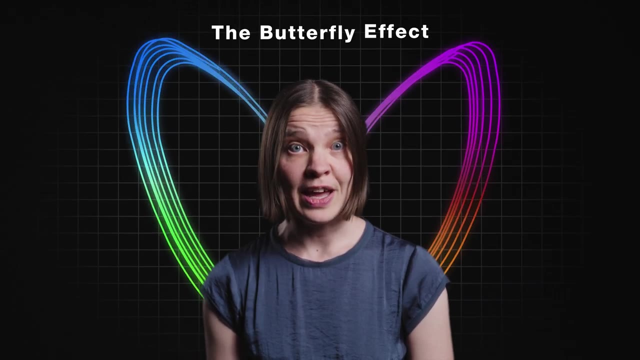 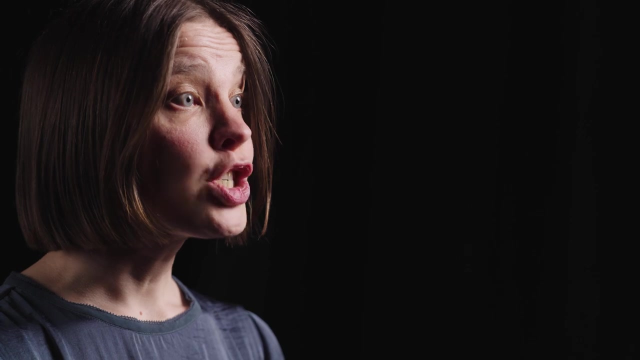 – explaining the equations that govern ocean waves and atmospheric conditions from fundamental principles. The most well-known illustration of chaos theory is, of course, the butterfly effect, conceived by mathematician and meteorologist Edward Lorentz in 1972.. It suggests that something as tiny as the flap of a butterfly's wings in Brazil could 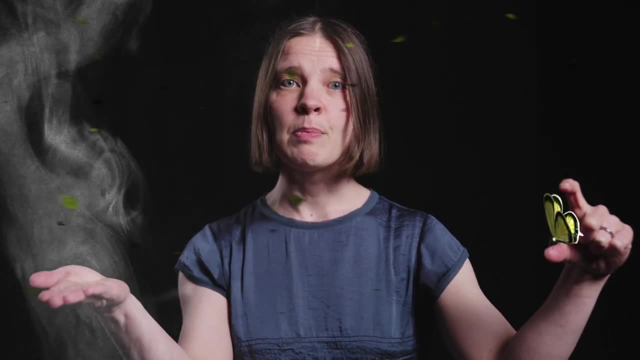 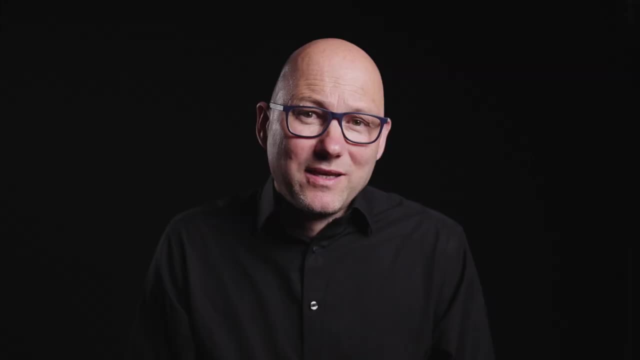 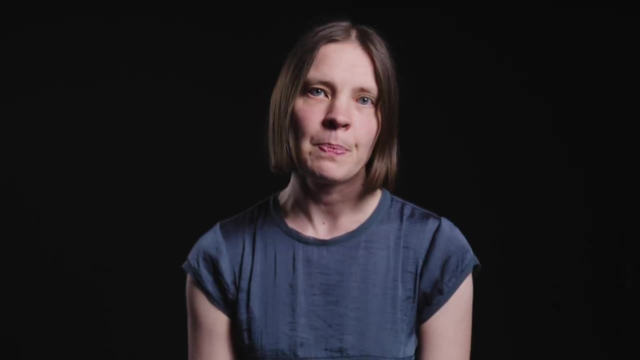 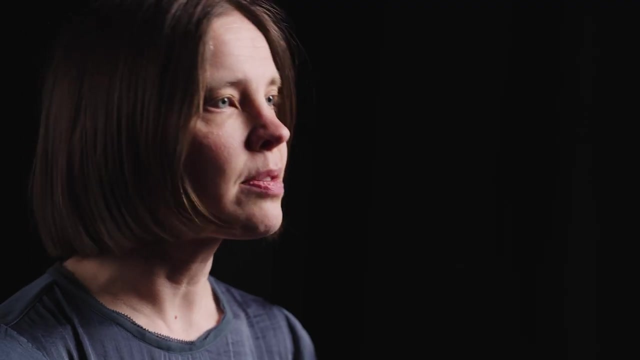 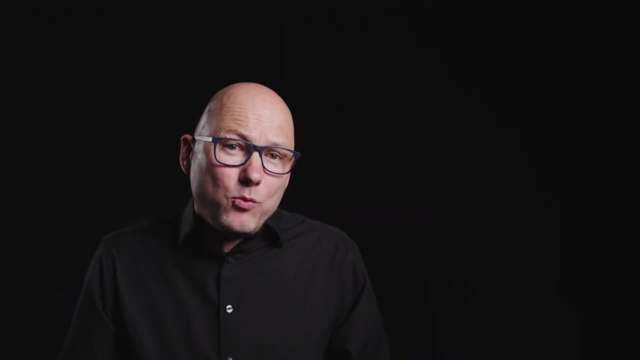 underlying a system this complex. Again, the law of large numbers comes into play, allowing us to predict the probability of a tornado caused by a butterfly. This is extremely unlikely – virtually impossible. You would be more likely to win the lottery a million times in a row. 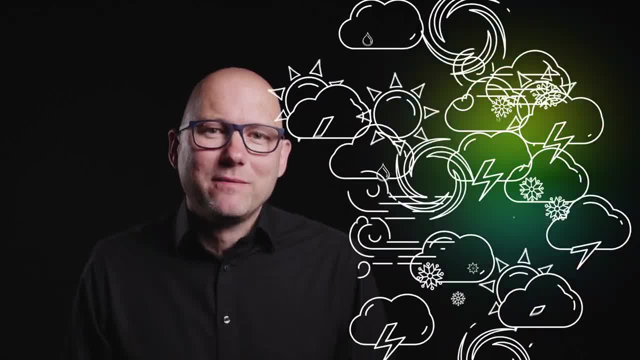 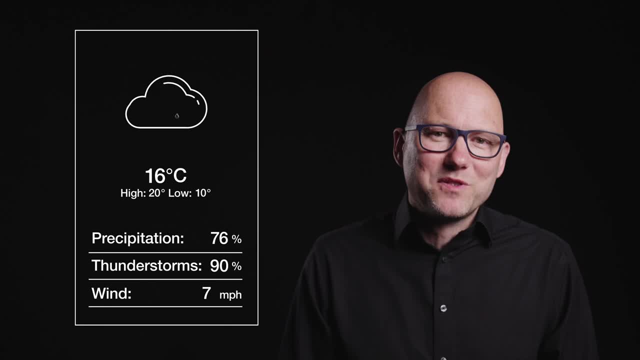 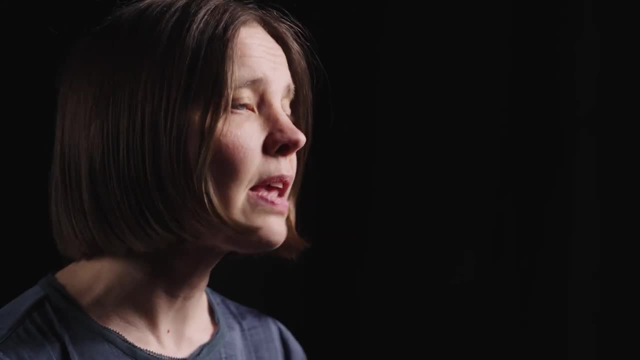 Similarly, we cannot predict exactly what tomorrow's weather will be, But we can make smarter weather forecasts that tell us the probability of a specific weather types with improved reliability. Understanding the mathematical foundations of chaos is important because this gives us practical insight into the complex systems behind major global challenges. 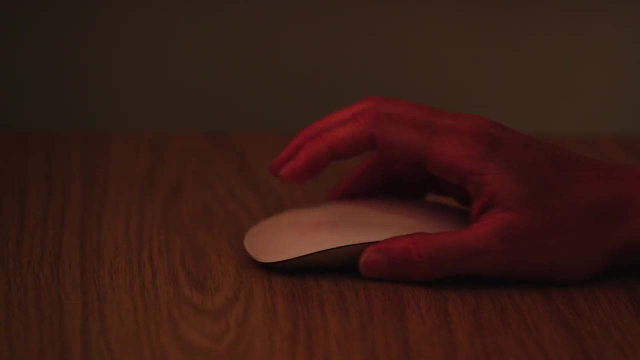 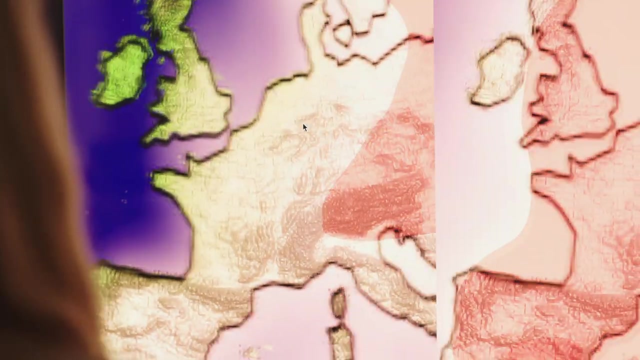 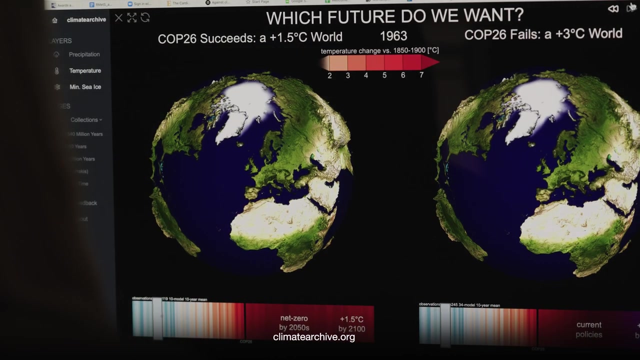 and provides the basis for new technological applications. For example, here at Bristol, our researchers are working closely with the Met Office and using novel approaches such as high-performance computing and machine learning to improve the accuracy and value of weather, climate and atmospheric models. This takes our fundamental knowledge of mathematics and physics.